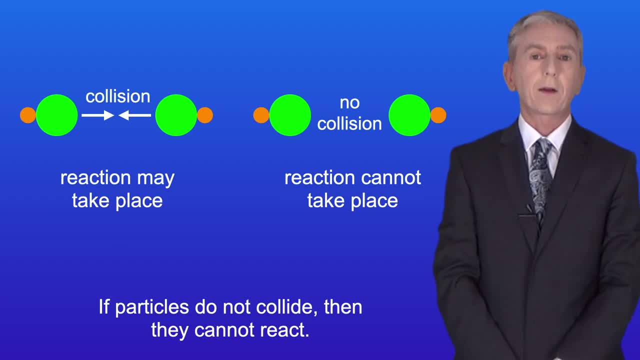 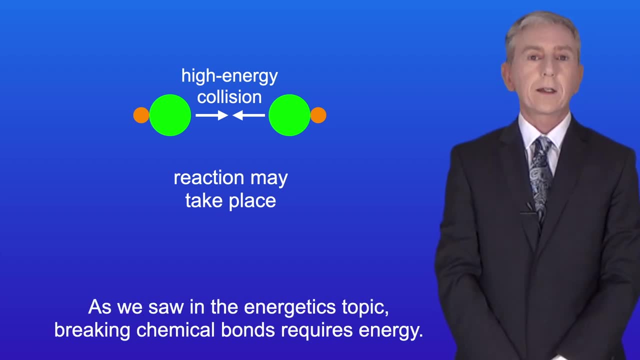 they must collide. If particles do not collide, then they cannot react. Secondly, when particles react, chemical bonds must be broken And, as we saw on the energetics topic, breaking chemical bonds requires energy, and scientists call this the activation energy. So, in order for a reaction, 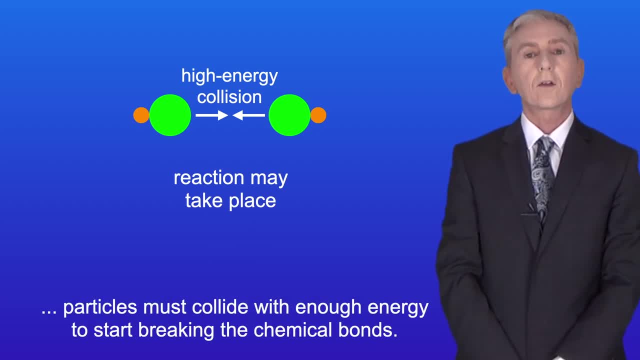 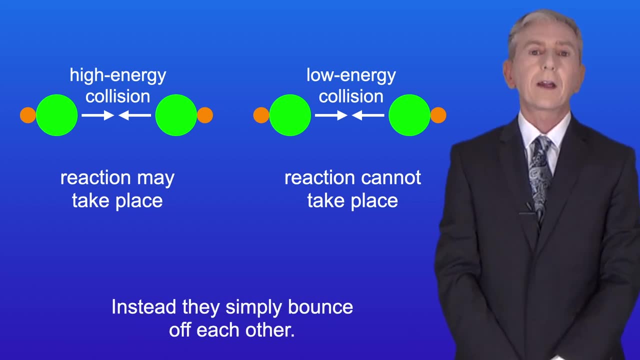 to happen, particles must collide with enough energy to start breaking the chemical bonds. If the collision does not have enough energy, then the particles cannot react and instead they simply bounce off each other. Now I should point out that we're going to be looking at activation energy in much. 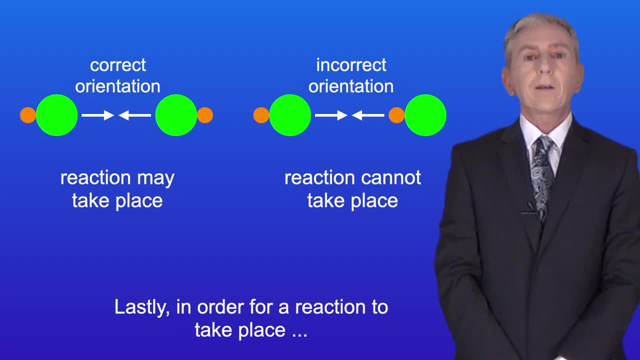 more detail in later videos. Lastly, in order for a reaction to take place, particles must collide in the correct orientation. In the reaction I'm showing here, the atoms in green must collide for a reaction to happen. So in the left-hand diagram the particles are in the correct orientation and a reaction 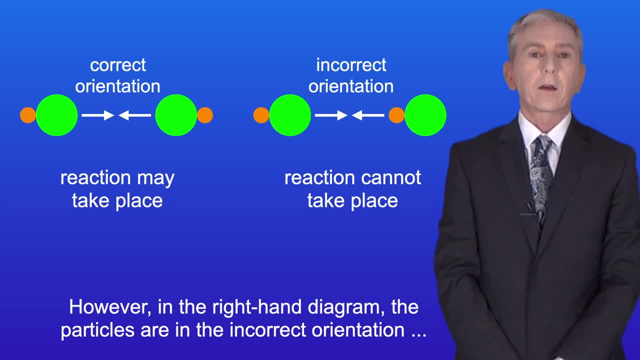 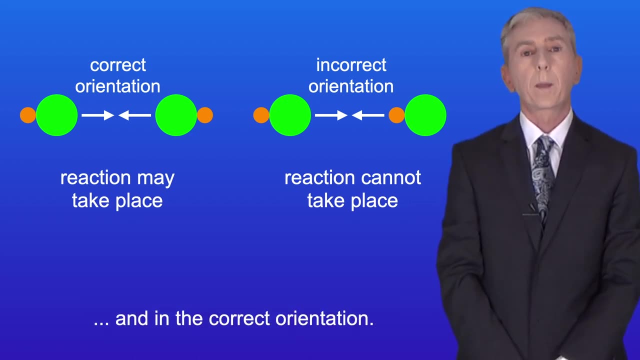 may take place. However, in the right-hand diagram, the particles are in the incorrect orientation, So this collision is ineffective and a reaction will not take place. So, in order to react, particles must collide with sufficient energy and in the correct orientation And the rate of 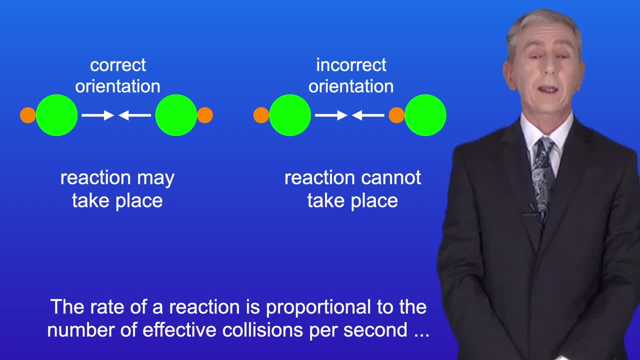 a reaction is proportional to the number of effective collisions per second, In other words, the frequency of effective collisions. Okay, now, one way to increase the rate of a reaction is to increase the concentration of the reactants, And we can explain that by using collision. 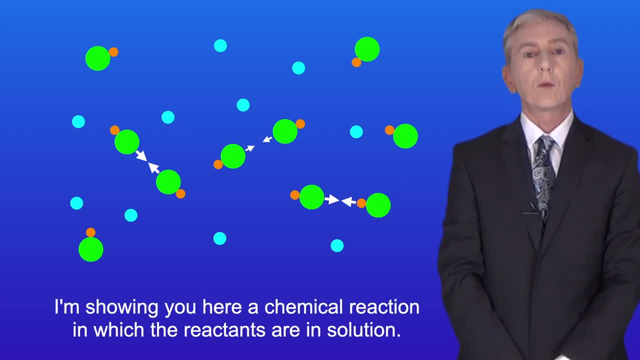 theory. I'm showing you here a chemical reaction in which the reactants are in solution And I'm showing the water molecules as light blue circles. As you can see, reactant molecules shown as A are not colliding, So they're not reacting. 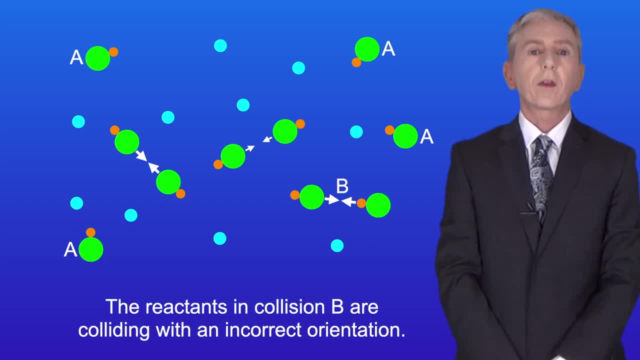 The reactants in collision B are colliding with an incorrect orientation. This is not an effective collision and a reaction does not take place. Reactants in collision C have the correct orientation And they're not colliding. So they're not colliding. So they're not colliding. 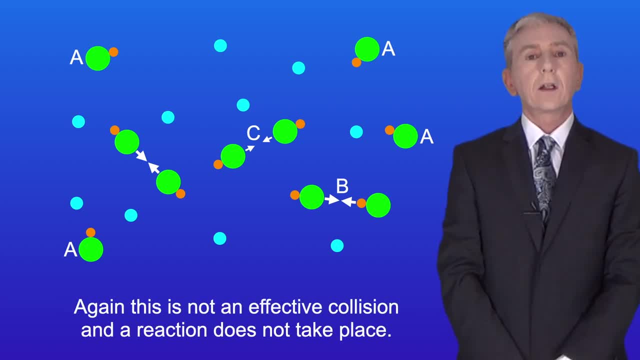 But insufficient energy. So again, this is not an effective collision and a reaction does not take place. Reactants in collision D are colliding with the correct orientation and with sufficient energy, So this is an effective collision and a reaction takes place. Now, as we said before, we can increase the